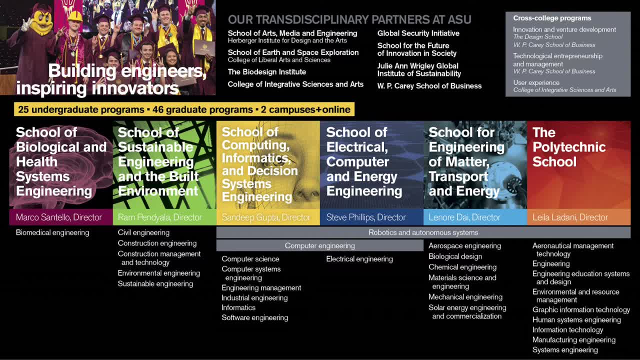 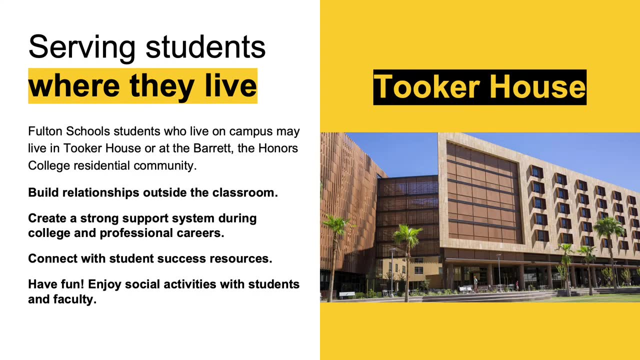 higher admissions criteria than the general university requirements. For a comprehensive list of admissions criteria, you can visit the Fulton website at engineeringasuedu. Students in the biomedical engineering program are located at the Tempe campus, which is both their academic and residential home. First-year freshmen are expected to live. 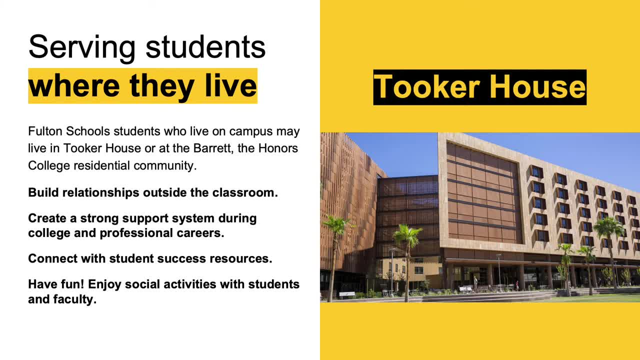 on campus their first year and our engineering students are currently registering for housing in the Tooker House. Tooker House is the residential hall for all of the engineering disciplines and we are also expanding to University House for the 2020-2021 academic year. Students that are a part 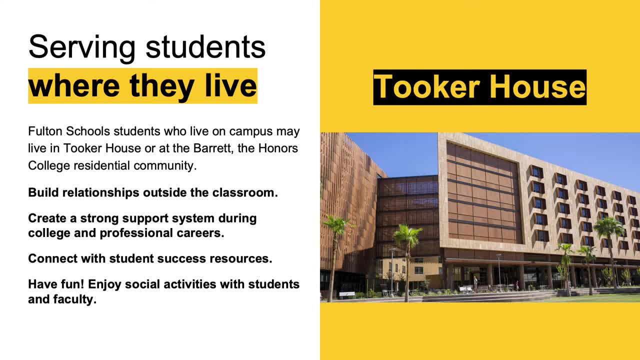 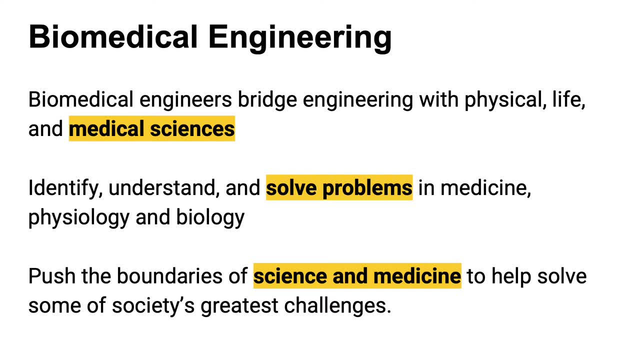 of Barrett, the Honors College, live in Barrett housing, but are given the opportunity to live on an engineering specific floor if they choose. Today, we are going to uncover what it means to be a biomedical engineer. Biomedical engineers are unique because they bridge traditional engineering with the other. 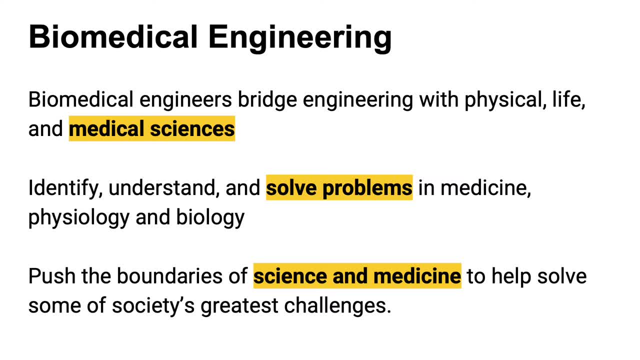 science disciplines, namely in the realms of biology and medicine. This is a rapidly growing discipline because of the rise of machinery and technology in all aspects of life and society, particularly related to health and wellness. Biomedical engineers are the first to live on an engineering-specific. 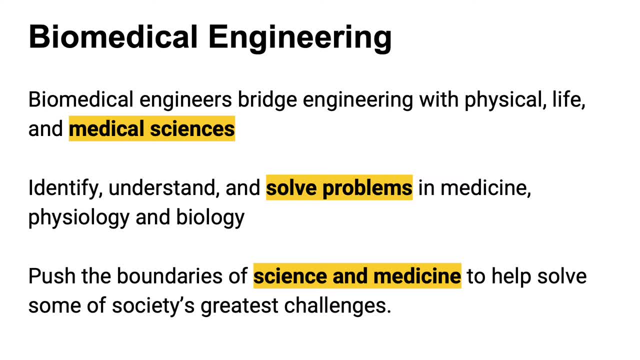 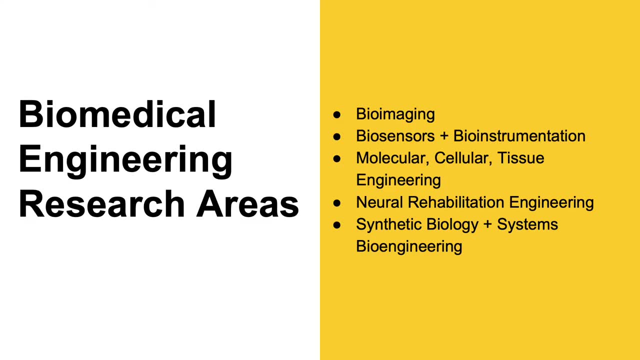 floor. Biomedical engineers work on everything from artificial organs and surgical robots to advanced prosthetics. This is an exciting field that pushes the boundaries of science and medicine to help solve some of society's greatest challenges. Faculty in the School of Biological and Health Systems Engineering. 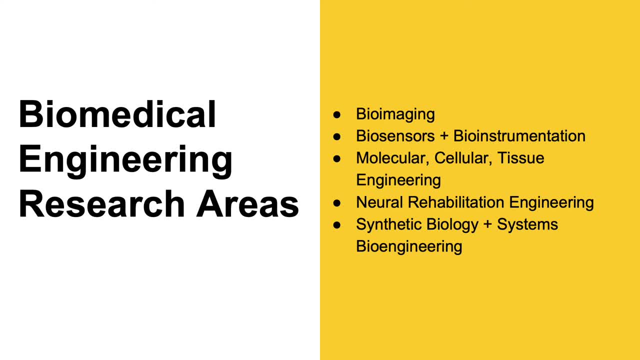 apply engineering principles and methods to understand, define and solve problems in medicine, physiology and biology. Our faculty seek to transform society through developing use-inspired technologies and getting those technologies into use through entrepreneurship. By its nature, our research is inherently multidisciplinary and the potential impact is global. The 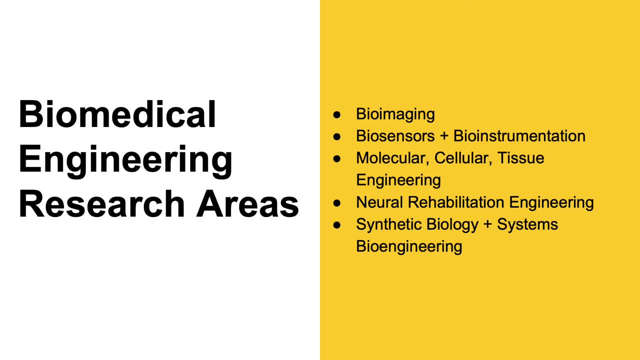 faculty in SVHSC have a wide range of research expertise and research interests and is particularly strong in the following research areas: Our imaging faculty work on developing new imaging techniques and contrast agents that target specific pathologies, creating translational imaging technologies and using novel MRI phase mapping methods to measure tissue electrical properties. 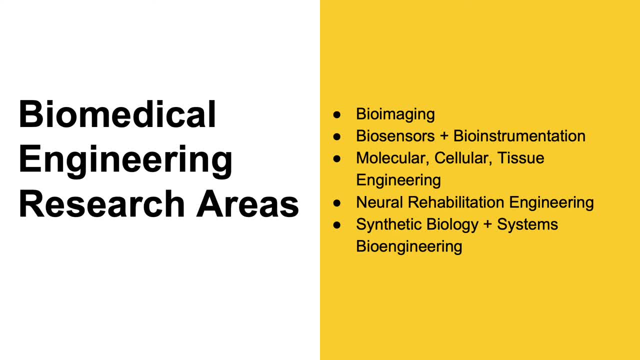 They collaborate closely with local medical centers across Phoenix, the Magnetic Resonance Research Center at ASU and the Keller Center for Imaging Innovation at Barrow Neurological Institute. Our biosensing and bioinstrumentation faculty focus their attention on research diagnostics for monitoring human and environmental health. They build microelectromechanical systems. 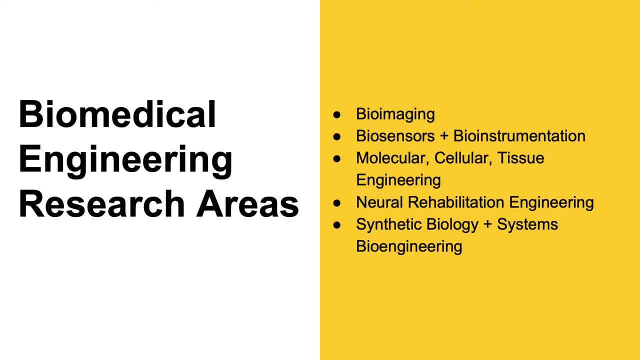 for better neural signal recording and drug delivery, and devices for interacting in real time with biological systems. Our molecular, cellular and tissue engineering faculty focus on novel biomaterials for rebuilding damaged tissue, molecular and cellular therapies and localized drug delivery systems for hard-to-treat cancers. Our neural faculty. 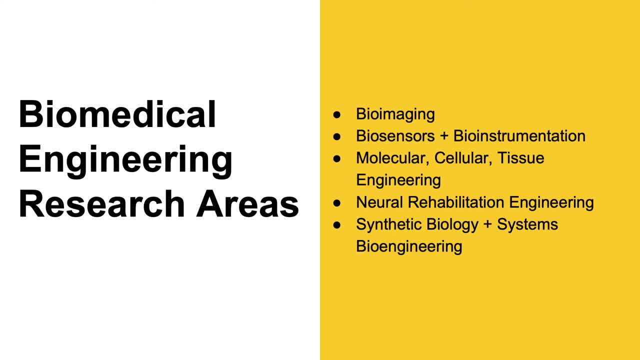 work on modeling and simulation of neural systems to gain insight into neural function, neural signal acquisition and analysis, and the development of specialized technology to evaluate and treat individuals with neural and biomechanical pathologies. The field of synthetic and systems bioengineering is based on the premise that living systems are modular and thus able to. 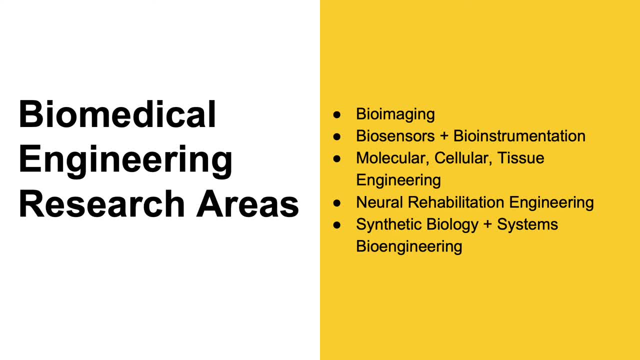 be engineered. This idea has spurred a new movement that has made a substantial impact on molecular and cellular health. Our biosensing and bioengineering faculty focus their attention on biological systems for better neural and cellular therapy. Our biosensing and biomechanical pathologies. focus on molecular and cellular therapy. This idea has spurred a new movement that has made a substantial impact on molecular and cellular therapy. Our biosensing and biomechanical pathologies focus on molecular and cellular therapy. Our biosensing and biomechanical pathologies focus on 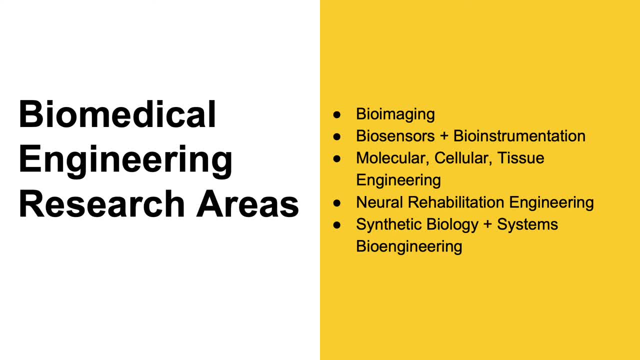 basic research, Synthetic and systems biology takes inspiration from the philosophical reflections of Feynman. quote: what I cannot create, I do not understand. In SBHSE, we design genetically encoded information and sell microenvironments to gain a deeper understanding of living things, as well as to generate useful products such as advanced 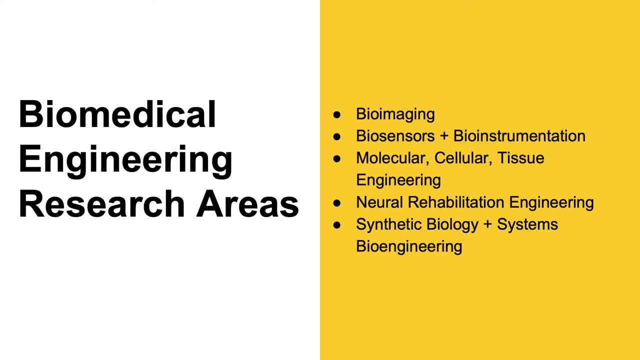 medical treatments. Here you will find research and coursework in engineering, bioengineering and biomechanical pathologies. Our biosensing and biomechanical pathologies focus on gene networks, policy and governments, biological network modeling and biomaterials for. 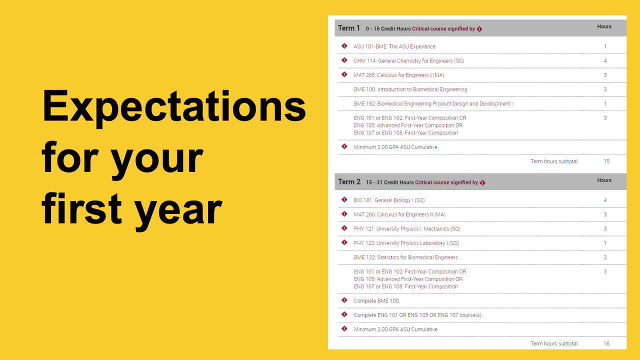 multicellular systems. Your first year in biomedical engineering is focused on developing a foundation in science and calculus. BME courses rely heavily on having a proficiency in math and physics, and your competency in these areas are predictors of future success. in the major, You can expect to take calculus, physics, chemistry and biology. 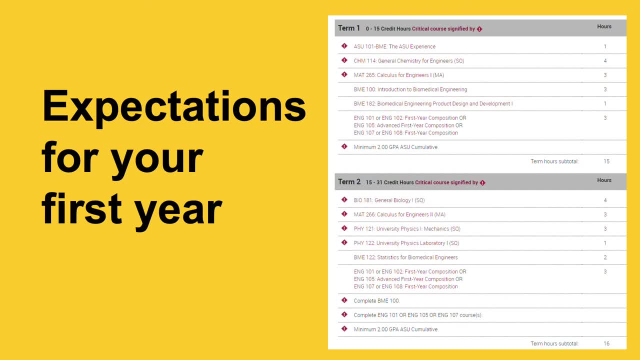 in that order. During your first semester, you will take BME 100,, which is an introduction to the BME industry and potential career paths, along with developing a better understanding of what engineers do and how to work in a team. BME 182 introduces the design process and is your first. 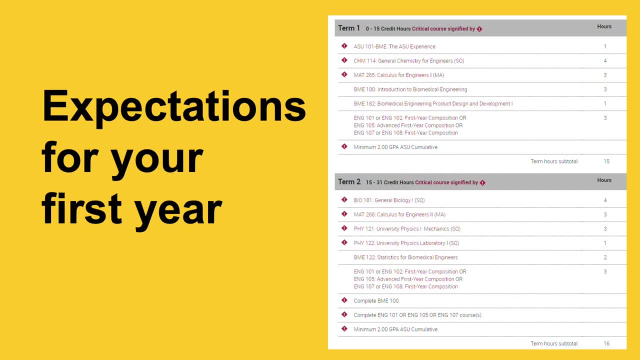 product design lab experience. This course further develops skills in collaboration and teamwork. All first-year students also take ASU 101.. As a BME student, you will also take ASU 101. as a BME student, This will be your first chance to interact with BME faculty and learn about BME. 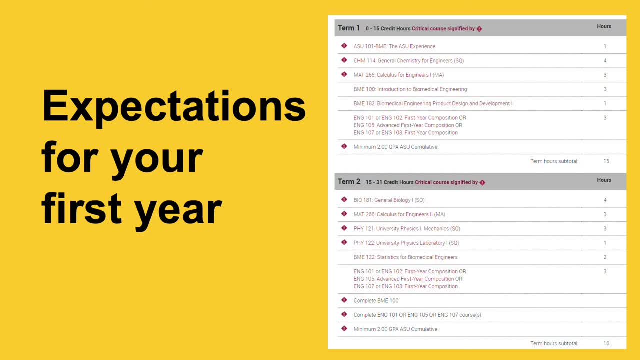 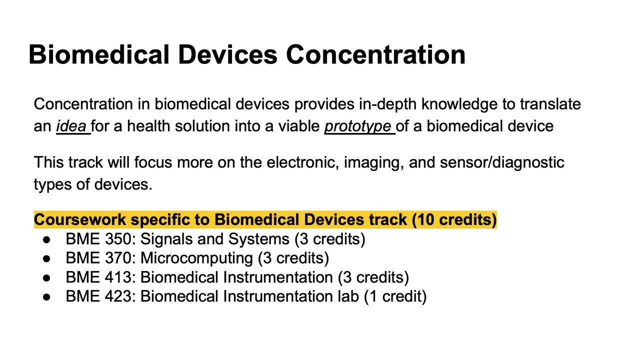 research areas. This course will also teach you the keys to succeed and thrive in your first year of college. The biomedical engineering program offers students two total concentrations: biomedical devices and biological devices. The biomedical devices track provides students with an in-depth knowledge to translate an idea for a health solution into a viable prototype. 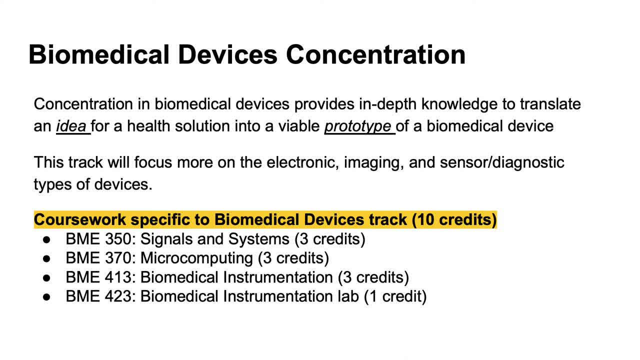 This track will focus more on the electronic imaging and sensor diagnostic types of devices. The difference in concentrations will appear in the student's fifth semester or the beginning of their third year, in which students in the biomedical devices track will complete 10 credits relating to signals and systems, microcomputing and the biomedical 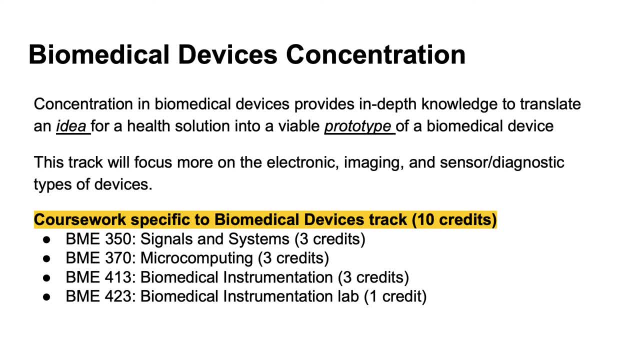 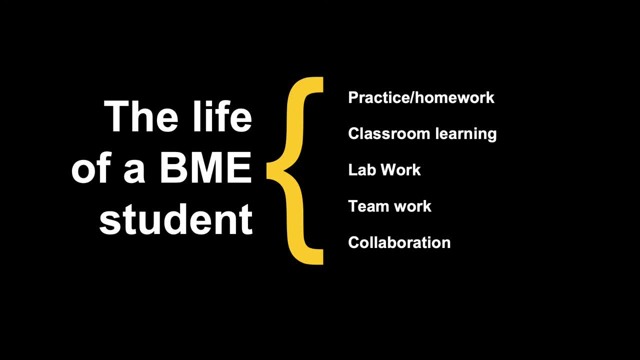 instrumentation, lab and lecture. The life of a BME student revolves around these core principles of BME. The BME students will be able to learn more about the BME research areas, While your specific activities will change between your first year and your senior year. 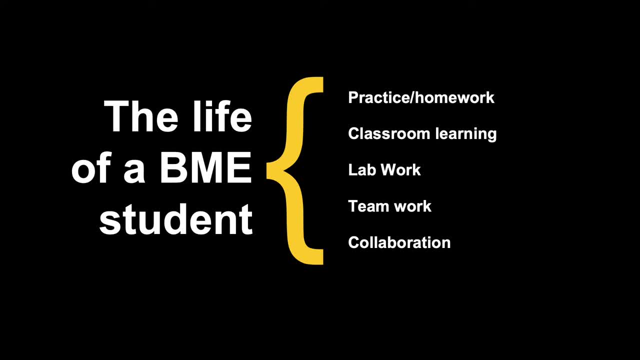 you can expect to engage in these activities throughout the time you are in this program. Practice makes perfect, and the homework you are assigned in your courses is not to torture you, but to help you practice the skills and content you are learning. There are many support networks available to you to help you succeed on your homework. 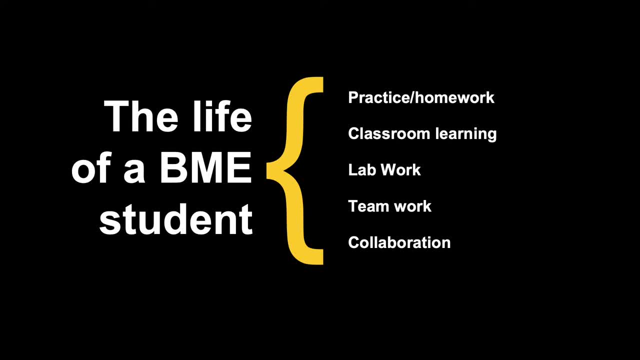 Fulton has two tutoring centers and there is no stigma whatsoever about attending tutoring. In fact, there is no stigma whatsoever about attending tutoring. In fact, there is no stigma whatsoever about attending tutoring. In fact, there is no stigma whatsoever about attending tutoring. 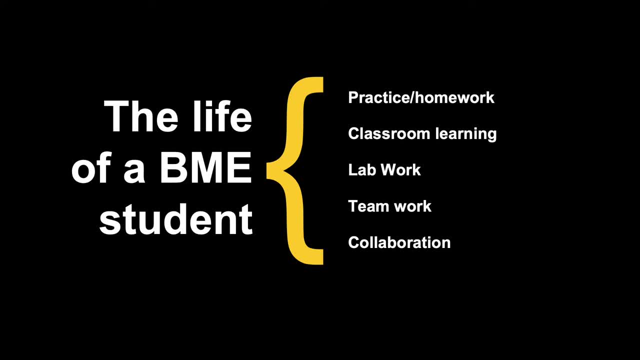 It is highly encouraged. Your learning will primarily take place in the classroom and the lab. These are the arenas in which you will gain the content as well as the practical skills needed to succeed in this discipline. You will be assigned team projects and learning to work productively. 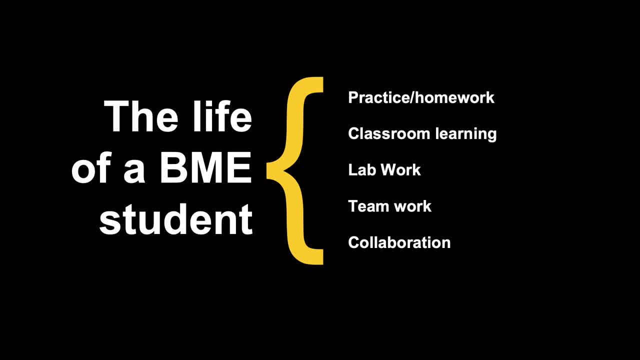 as a member of a team is one of the greatest skills you will learn as an undergraduate. You will need to balance your academic activities with all of the other fun and exciting things going on around you. Planning ahead is key. You will need to balance your academic activities with. all of the other fun and exciting things going on around you. Planning ahead is key. You will need to balance your academic activities with all of the other fun and exciting things going on around you. Planning ahead is key. You will need to balance your academic activities with all of the other fun and exciting things going on around you. 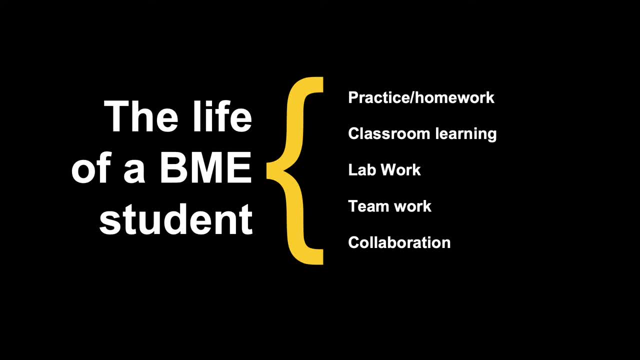 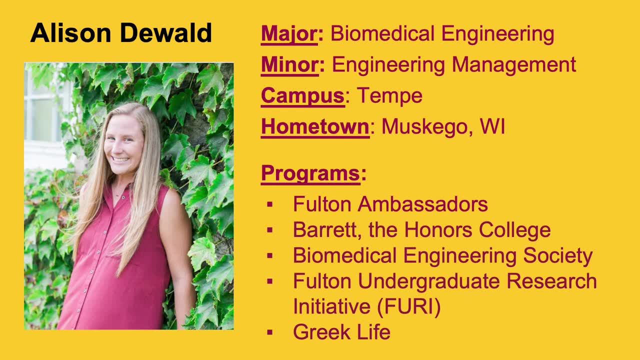 And your faculty. academic advisors, peer mentors and friends are available to assist you. Hi everybody. my name is Allison DeWald. I am a current junior studying biomedical engineering with a minor in engineering management. I am based off of the Tempe campus. 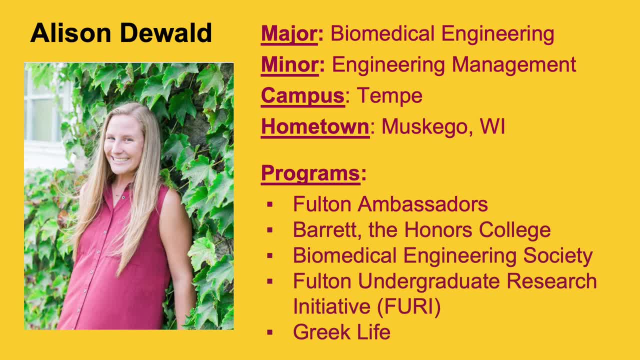 I am from a small town in Wisconsin, so I'm an out-of-state student, but it was definitely one of the best decisions that I've made to decide to go to ASU. Just going over a couple of programs that I'm involved in on campus, I am in Fulton. Ambassadors, which is a leadership organization on campus that does recruitment and outreach events. Just going over a couple of programs that I'm involved in on campus: I am in Fulton Ambassadors, which is a leadership organization on campus that does a lot of recruitment and outreach events. So things like this or other events that are held on campus are just some things that we volunteer for. I'm also in Barrett-The-Honors College. I'm currently doing my thesis with Cameron, who will be introduced on the next slide. I am in the biomedical engineering society, which is one of the engineering-specific 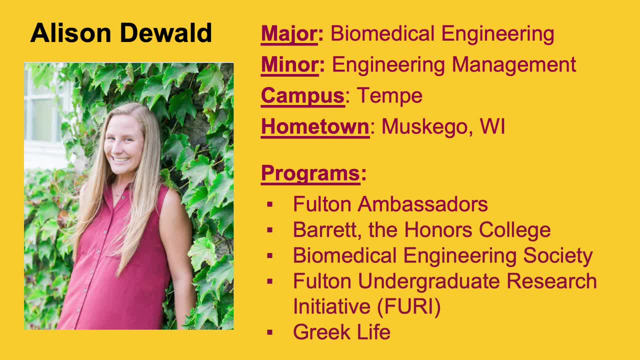 clubs that we have on campus. currently, Where we plan behind the scenes is where we'll do an internal yahoo page campus. You don't have to specifically be a BME major to participate in the club, but it is really great. We reach out to a lot of industry professionals as well as professors. They come 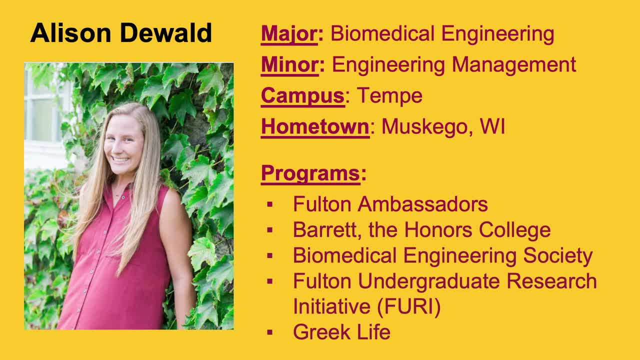 in talk about their research so you're able to kind of see a glimpse into the future of what this major could hold for you. I'm also currently doing undergraduate research for my thesis, so I'm doing it with a doctor over at Dignity Health and I'm doing some research regarding pressure ulcers. 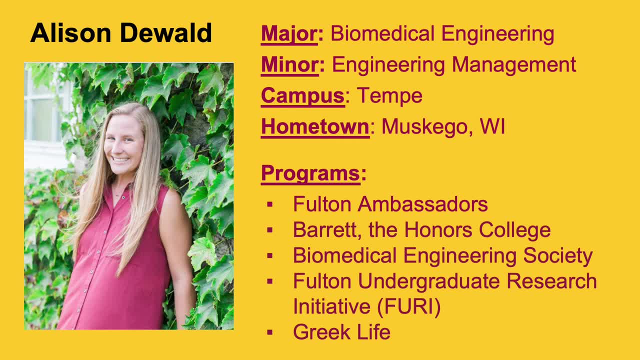 and pelvic binder projects. And then I'm also in Greek Life, which is an organization that is non-academic. It's a really great opportunity for meeting people and continuing any volunteer that you might have previously done in high school, as well as just having some like more fun things to. 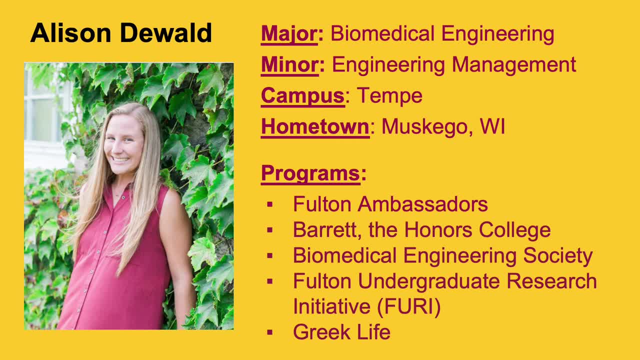 do in your free time that aren't related to engineering specifically. So getting into why I decided to join BME. So something really interesting about BME is that it's a really cool that my high school did was we had to complete a research paper on what we thought. 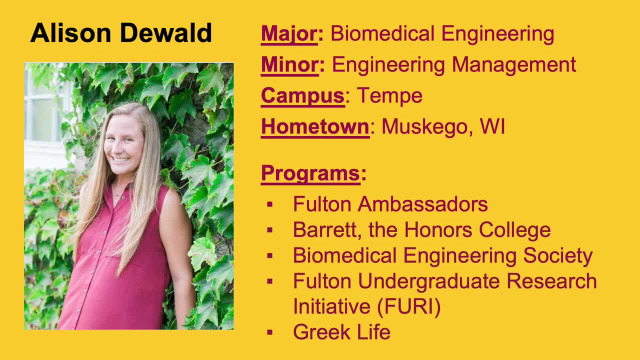 our future profession was going to be, And I actually heard about biomedical engineering from one of my parents' friends. It kind of mixes together both of my parents' professions, So my mom's in the medical field and my dad works with computer engineering. So it was a really 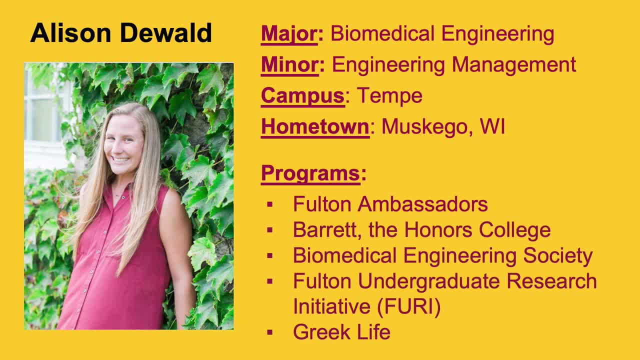 great opportunity for me to kind of use my strengths in what I choose for the future. So I ended up writing my research paper on biomedical engineering and I did a job shadow. I ended up job shadowing a biomedical engineer. He graduated from Marquette, which is a university. 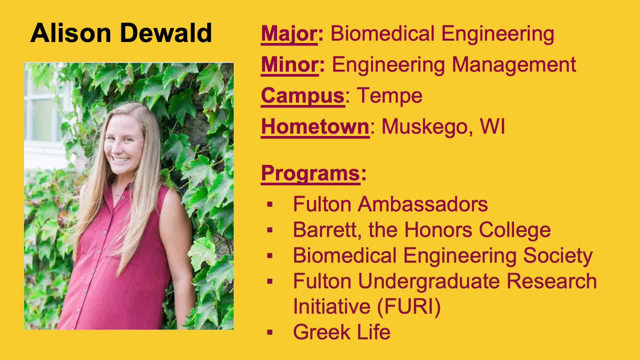 in Wisconsin And he works with people who suffer from epileptic seizures And he uses electrodes to target specific areas on the brain and then studies where, why, how those seizures are occurring and then hopefully help them find a way to combat those seizures in the future. So after I did that, 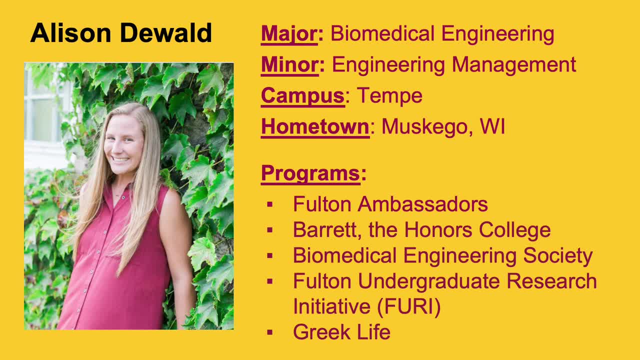 job shadow, I kind of realized that this is something I could really see myself doing in the future. And then, as I progressed through courses- I just am further trying to think of the correct word here- told or like shown that this is something that I wish to pursue in the future. Another: 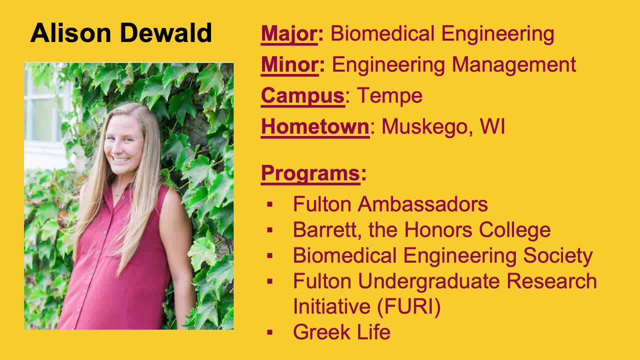 great thing is that there's a lot of opportunities of what you want to do. A lot of students might go to med school on to do a PhD program, Some go to law school or you can go directly into industry and having that option as an incoming freshman to know that whatever I wish to pursue, I was going. 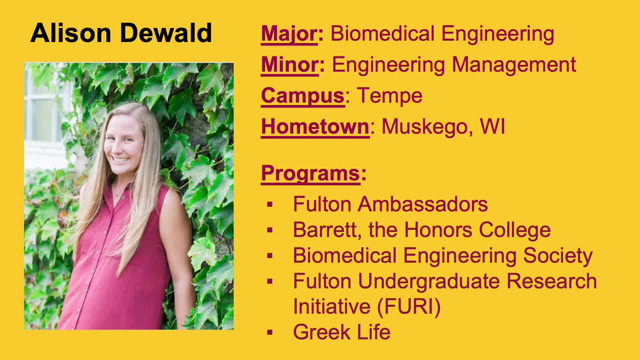 to be able to do So. I'm going to be able to do that. So I'm going to be able to do that. So I'm going to be able to do love in medical chemistry. I'm going to be able to do models. that's something. 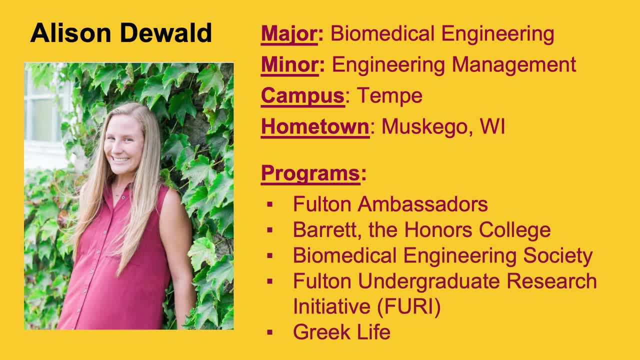 I Sab�� to do was something that really stood out to me. on the typically do on the special ed, to do was something that really stood out to me, excuse me. So of the courses that I really enjoyed over my time, a lot of my BME specific courses, So as you go through you might have someore gen. 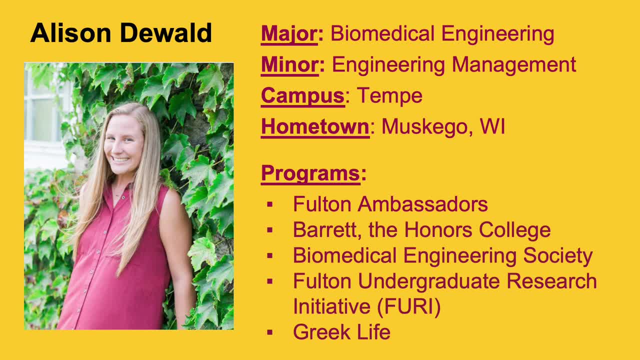 He had had. I don't really wanna call them jetus because they really do relate to your degree, but like physics or chemistry. But once I started getting to where then is program and really see what I'm able to do in the future with my profession, 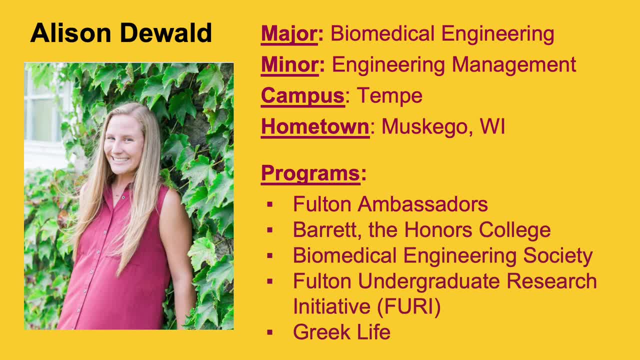 As far okay, so I've gone through what I'm involved in. Something that might be helpful for you guys to hear is that it's okay to change your major in college. A lot of students do it and I have a lot of friends who were in VME their freshman year and decided to switch out. 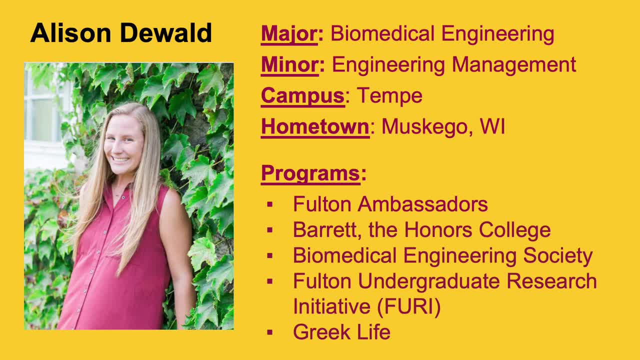 But a really great thing that ASU offers is a lot of different programs. So, regardless of whether or not you want to pursue engineering or biomedical engineering specifically, you will have that option and that flexibility within this university to really find what your niche is and 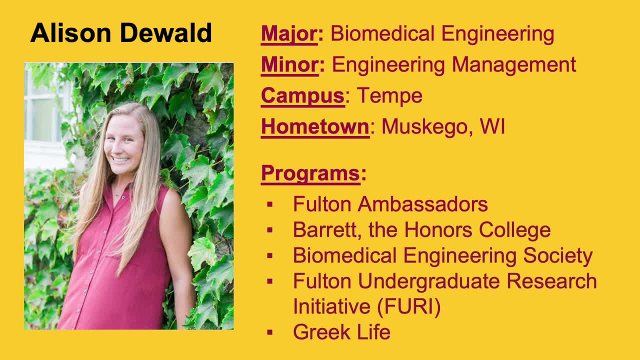 what interests you, And I think that that is a really great opportunity for you to know that you're choosing a university that has a lot of options for you to pursue whatever it is that interests you the most. So, yeah, that's it about me, and then I will pass it off to whoever's on. 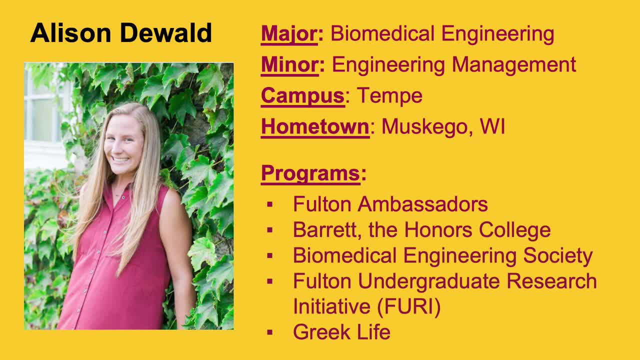 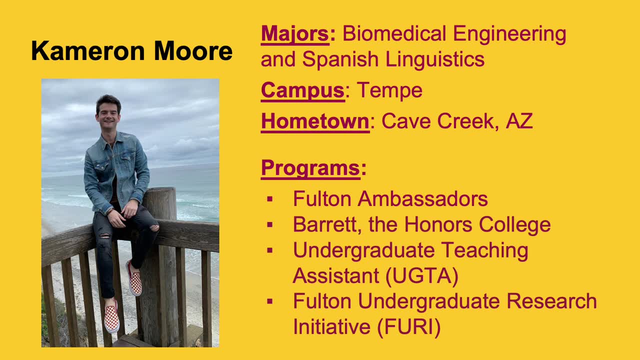 the next slide. Bye, guys, Good luck. Hi there, My name is Cameron Moore. I am a current junior studying biomedical engineering and Spanish linguistics. I'm pursuing concurrent bachelor's degrees and I wanted to talk a little bit about my experience at ASU and how I chose my majors. So I always wanted to do something that. 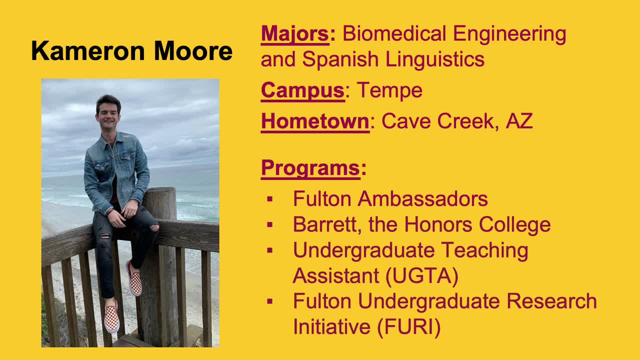 had to do with technology and healthcare, but I wasn't quite sure what avenue I wanted to take. I thought about working with a major that was something more biological, biologically focused, but then I found myself craving more technology, So I decided to try out. 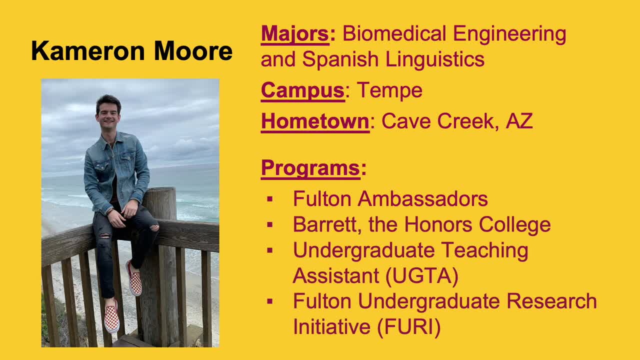 biomedical engineering. I originally started in the pre-medicine track as I was interested in going to medical school, but then I really fell in love with the technology and the ability that ASU has for students to develop their passion through technology and through device design. 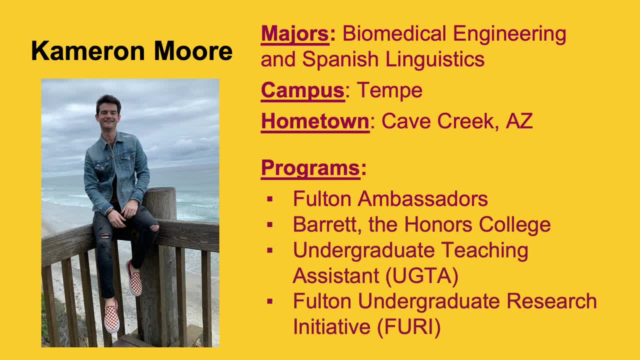 and engineering. So I really fell in love with the technology and the ability that ASU has for students to develop their passion through technology and the ability that ASU has for students to develop that strong connection with my degree program And I ended up taking myself out of the pre-medicine. 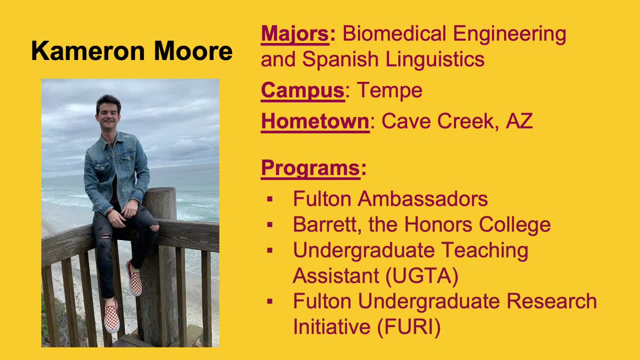 school track and then also pursuing my interest in studying Spanish as a world language. So I am pursuing two bachelor's degrees in that And my goal, my hope, is to work for a healthcare organization that focuses on international healthcare and healthcare education. So I'm 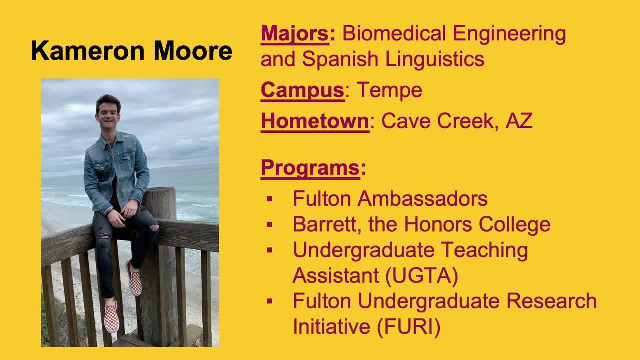 pursuing two bachelor's degrees in that, And my goal, my hope, is to work for a healthcare organization that focuses on international healthcare and healthcare aid. Something such as the World Health Organization or Doctors Without Borders are some career paths that are very appetizing to me. 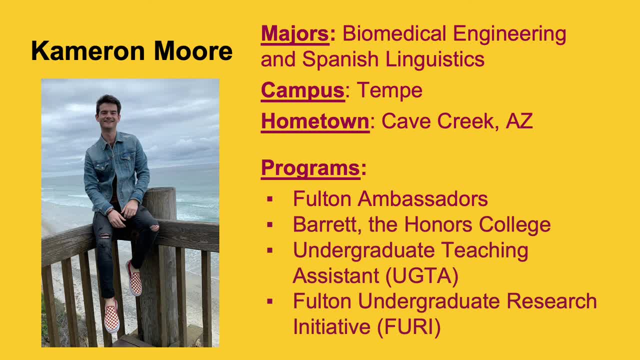 Something such as the World Health Organization or Doctors Without Borders are some career paths that are very appetizing to me. Hopefully it works out for me. So far in my degree program I've really really enjoyed how my classes have given me hands-on experience. 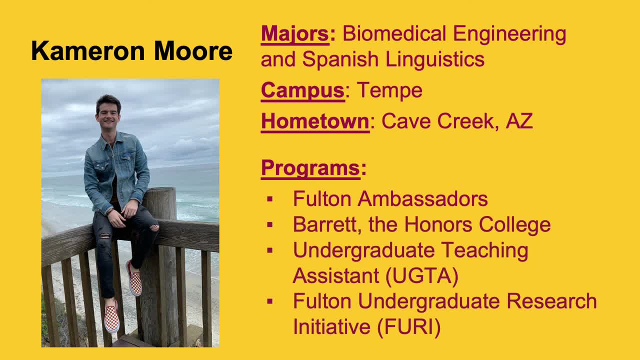 especially in my physiology lab. We learned so much about the body, both in humans and in animal subjects, and we learn about How different systems work with each other through different ways that they can interact with each other. So I'm really excited to be at ASU and I hope that you'll brings a healthy, healthy, healthy environment for everyone. 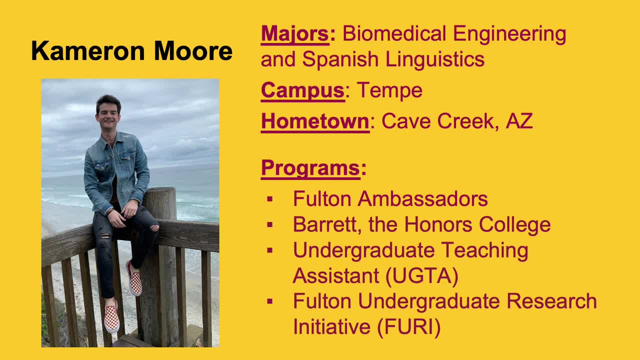 Thank you for your time hands-on laboratory experience. I've also really enjoyed working with some of our other courses that are less spoken about, such as conservation principles. I feel that class BME 200 is one that is essential to understanding a lot of the higher level physics and biology and chemistry that goes. 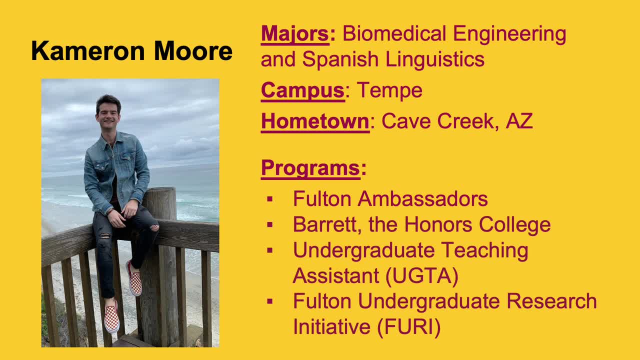 into biomedical engineering as well, as it introduces us to a lot of mathematical simulations and modeling and learning how to use tools such as MATLAB in our careers- Some programs that I'm involved in outside of my degree. I am a member of the Barrett Honors College. 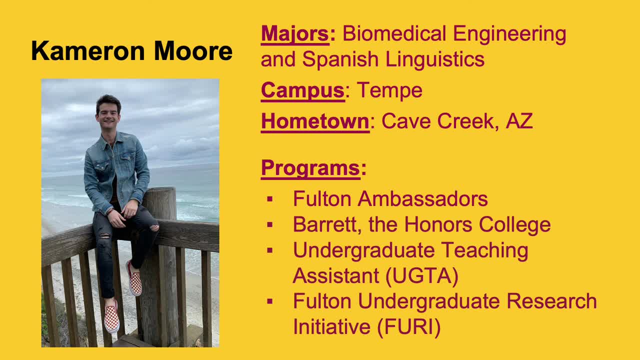 I am a Fulton Ambassador, which is the group that I'm speaking to you with now. It's a paraprofessional organization that allows students to make connections with prospective students, alumni, current students, and it is a really engaging program for people who like to communicate and 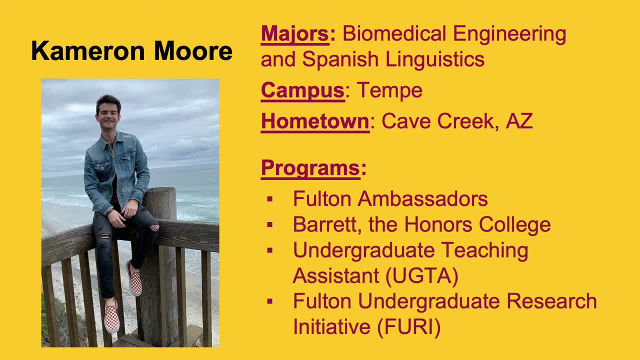 share their ideas with other people. I've also. so I'm an Arizona native and I grew up in Cave Creek, Arizona, and I wanted something that felt close to home for me but also far enough away that I had my own space, and I definitely felt that with ASU It helped me a lot, gained my 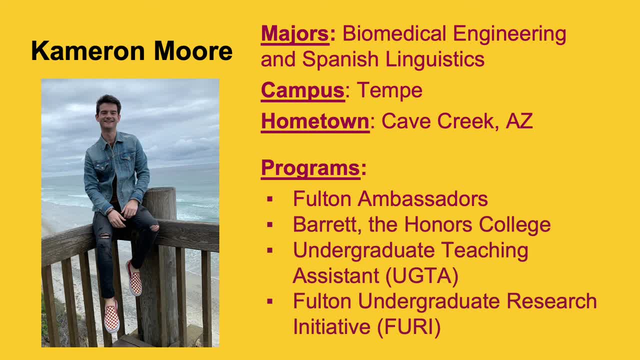 independence, I think, and ASU. they really do try to focus not only on your scholastic experience in the classroom, but also your holistic experience at ASU, which I've really, really thoroughly enjoyed between all of the events that they have for first-time students and all the other students as well. 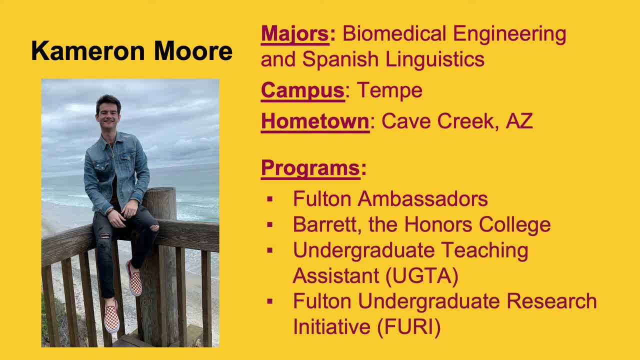 and the amenities that are available to students. resources such as office hours, TA ships, things like that I've definitely taken advantage of. I'm an undergraduate student, so I have my own space, I have my own time. I have my own. 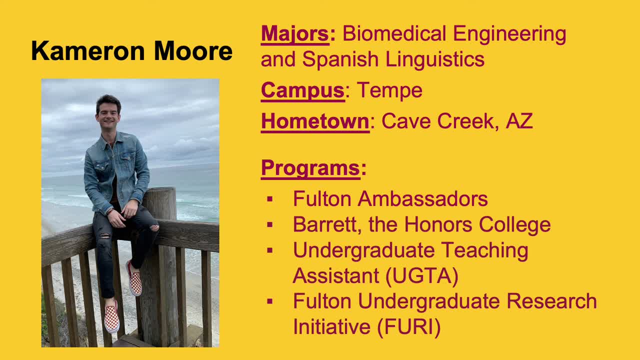 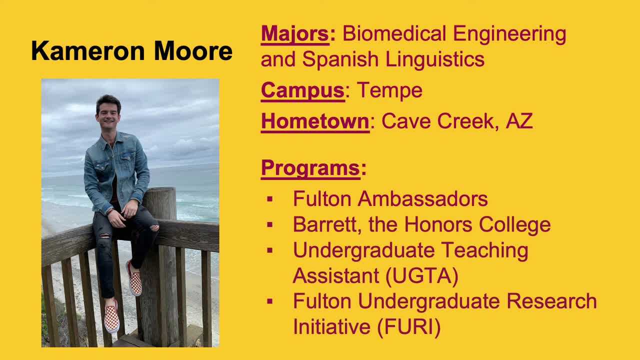 learn so much better the material from that course and other courses through teaching. Well, thank you so much for listening to my little story. I really look forward to meeting you and I hope that you choose ASU and engineering as your career. Thank you so much. Have a nice day. Hi, I'm Lexi. I'm a junior in 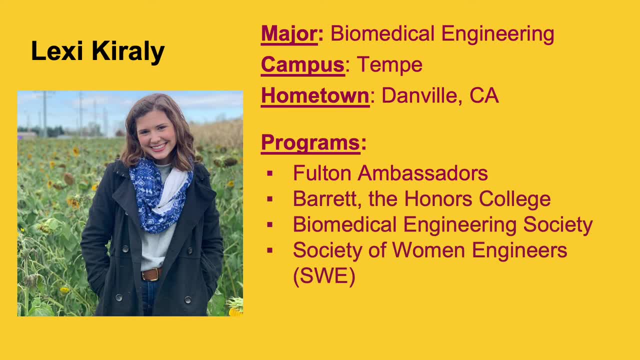 biomedical engineering here at Arizona State. I am involved in a few organizations, some of which are Fulton Ambassadors, and I have been involved in Fulton Ambassadors since I was a freshman and these last three years have been so much fun working with such talented engineering students and the 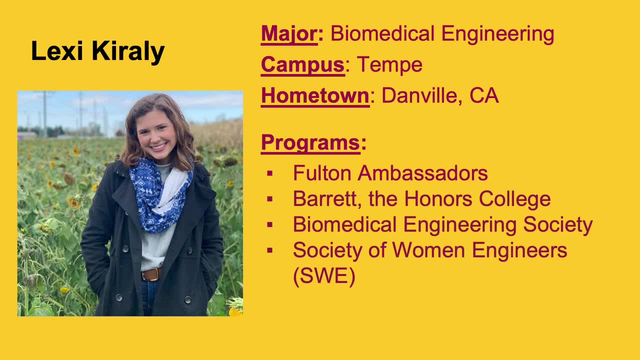 amazing recruitment staff. We get to put on special events and host a lot of events. We get to have a lot of fun and we get to have a lot of fun. We get to have a lot of fun and we get to have a lot of fun. We get to have. 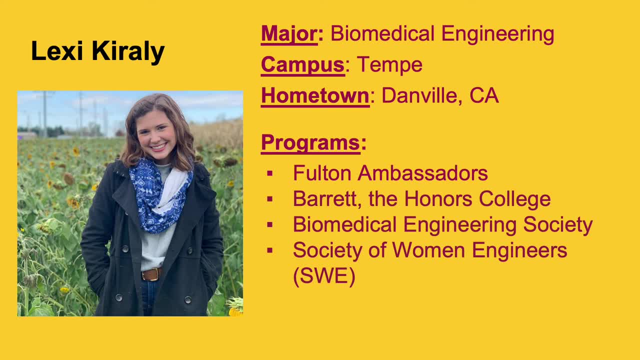 tours, and it's truly such a fun experience. I'm also in Barrett, the Honors College, the Biomedical Engineering Society and the Society of Women Engineers, and each of these organizations is so unique and they've really allowed me to grow not only as a student, but as an individual for the 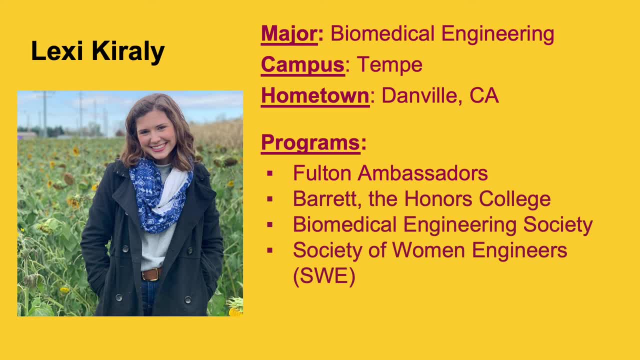 challenges that we tackle together and the solutions that we find. Some of the courses that I've really enjoyed over my journey in particular are organic chemistry, anatomy and physiology, biomaterials, microcomputing applications and biomechanics. And the cool thing about these courses in 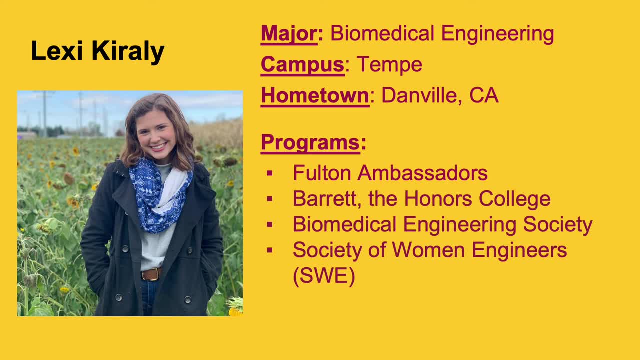 particular is that they each have supplemental lab sections where you're actually able to practice the skills that you learn in lecture. So not only are we being taught these concepts by such talented professors, but then we're actually able to practice the skills hands-on in the laboratory. 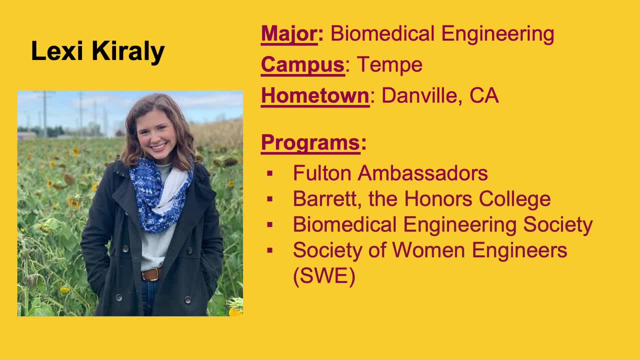 environment, which is probably why I've enjoyed the courses so much, And you also get to build such great relationships with your professors. They're there to help you and to teach you and they really just want to see you grow, And that's how I actually discovered who I wanted my thesis professor to be through 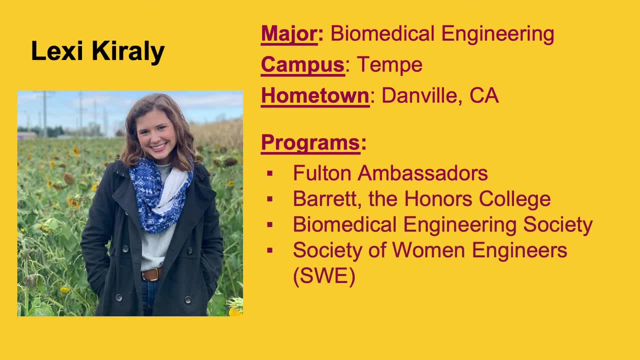 one of the courses that I took earlier on this year And I'm really excited to say that I am now involved in research that revolves around this course And I'm very excited to continue learning and growing and challenging myself with this research. So I chose BME because I really wanted to bridge the 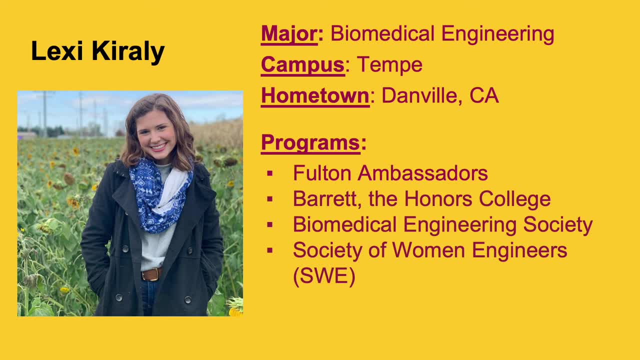 path between what I love and helping others. I wanted to problem-solve and be a part of something where I believed I could make an impact. That was a really big motivation for me- that I felt like I could benefit other people And I love. 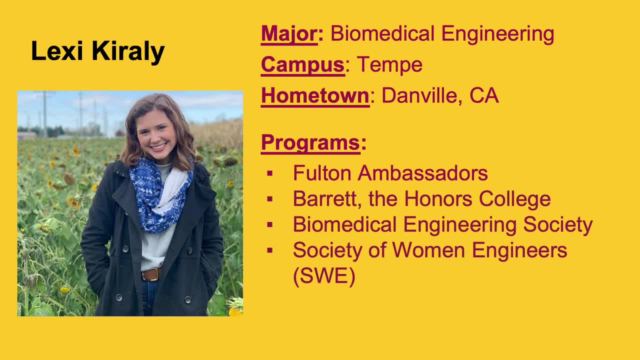 that the program at ASU does this, but the program itself isn't as easy as it seems. So if you are learning and you're interested in this, and you're interested in a course, because they merge the technical engineering work with the hands-on biological practice, 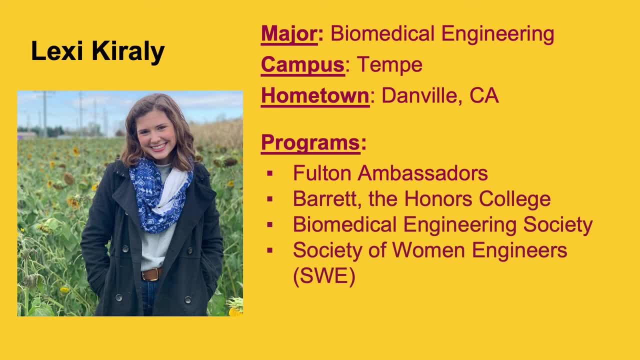 We're allowed to be as creative as we want with things like design projects. for example, In the lab work that I mentioned previously, we get to apply the skills that we learn to these real-world examples and problems that need solving, And there's so many skills that I've obtained throughout my relevant coursework. 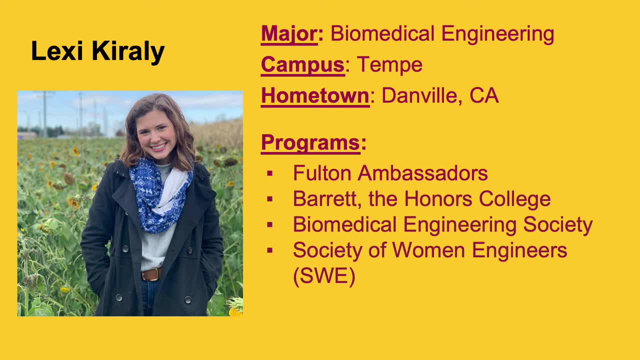 I feel like my analytical and communication skills have definitely grown. My creativity has grown, My mathematical and problem-solving skills have advanced, And there are so many places for these skills to be utilized in the workplace and different career paths that you can take on.